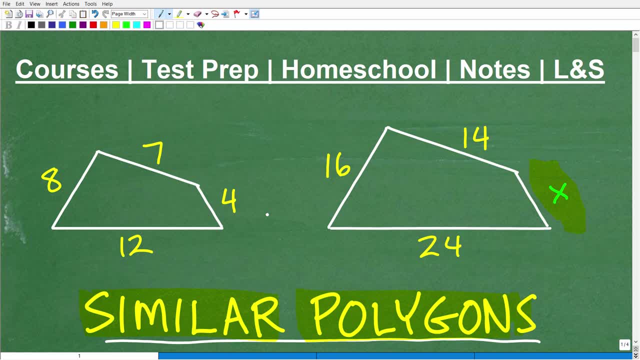 speaking to those of you that have a tough time with mathematics: Please do not give up. The number one thing you need to be successful in math is great math instruction, And what I mean by that is whoever you're learning math from, or whatever you're learning math from, it's got to. 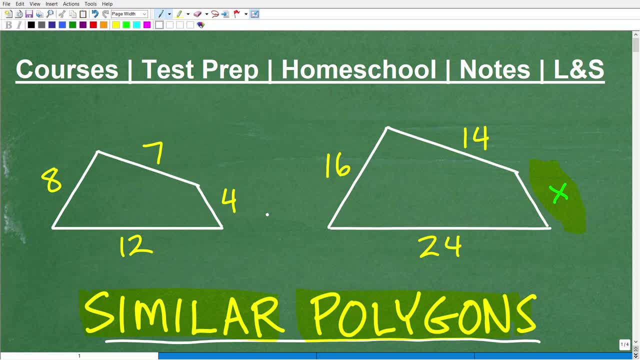 make sense, all right. Nothing's more frustrating than sitting in the classroom and being totally confused for an hour. And this is not a knock on any particular teacher. or maybe you're trying to learn math from a textbook, And if you're learning math from a textbook, you're going to have to. 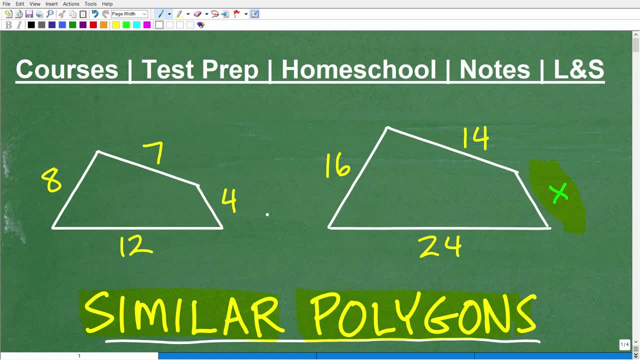 learn math from a textbook And you're just totally confused, right? If you're always confused, you're not going to learn math. See, math is a technical subject And sometimes it can be taught in an overly technical manner. The way I like to teach math is to explain things in an easy to 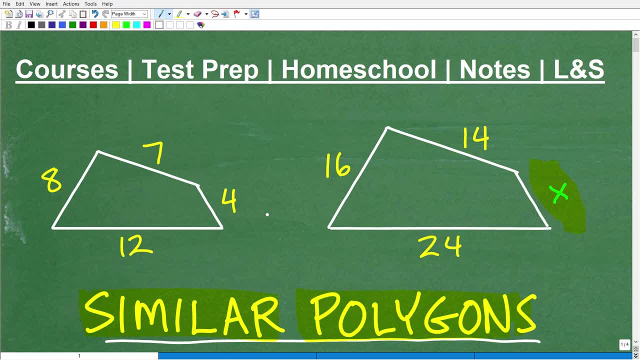 understand way so all students get what's going on without watering down what you need to know. So if you need help in your current math course or maybe some sort of special test that you're getting ready for that has math on it- I'm talking about things like the GED, SAT- maybe a teacher 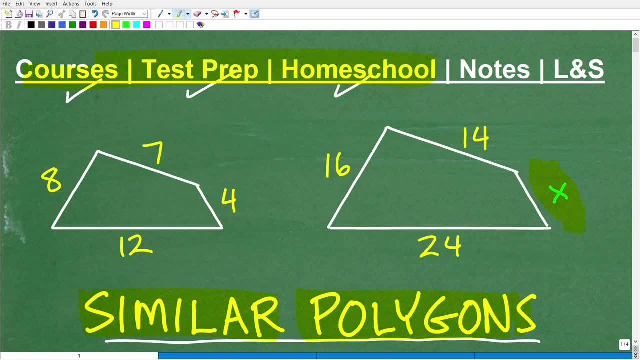 exam. or if you homeschool mathematics, check out my math help program. I'm going to leave a link to it in the description of this video. I literally have over 100 plus different math courses that span these categories and much, much more. I'm also going to leave links to my math notes in. 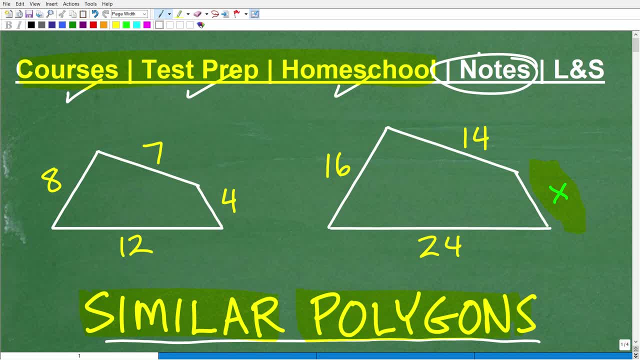 the description as well. You absolutely must be a great note taker to be successful in math. So if you're not taking notes or if you're taking so-so notes, improve your notes and you're going to see magic happen in terms of your grades. 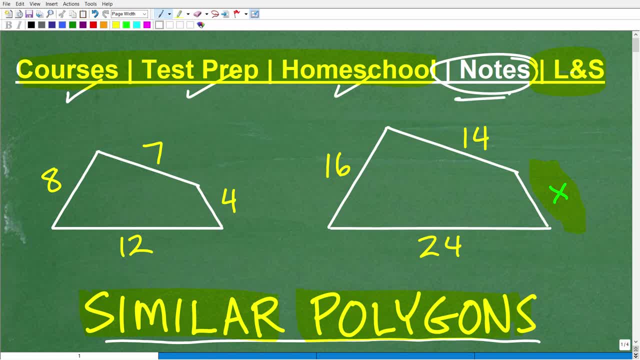 But, anyways, you can use my notes in the meantime if you like. And if this video helps you out, don't forget to like and subscribe, as that definitely helps me out. Okay, so let's talk about these words here real quick. It's similar in polygon. then I'm going to show you the right. 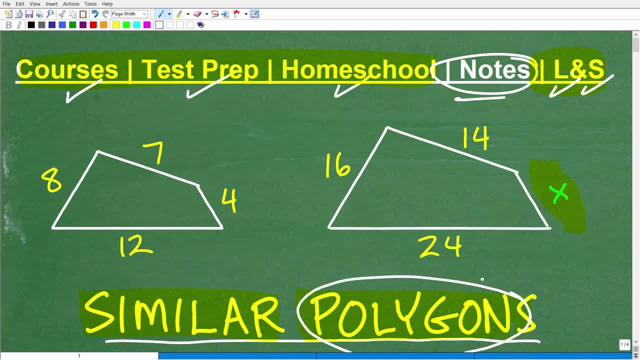 answer: A polygon effectively is just a closed figure made up of- I'm using very loose language here- of just like straight segments, okay, straight line segments. The first polygon we can have is a triangle. okay, then you can have rectangles or quadrilaterals, and then you can have. 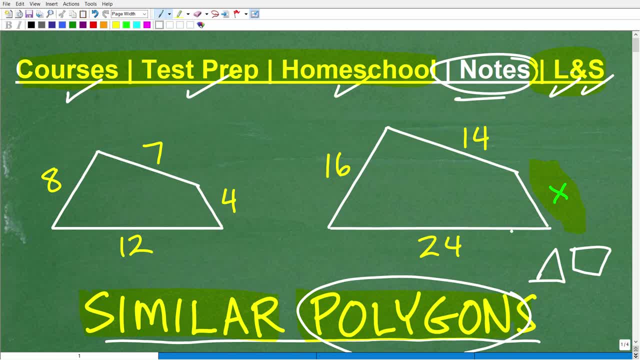 rectangles or quadrilaterals. So this is some sort of polygon. That's what a polygon is. And now similar? okay, well, the symbol for similarity is this little symbol. We'll talk more about what similar means, but just in case you were wondering what a polygon was, that's what it is And I'll 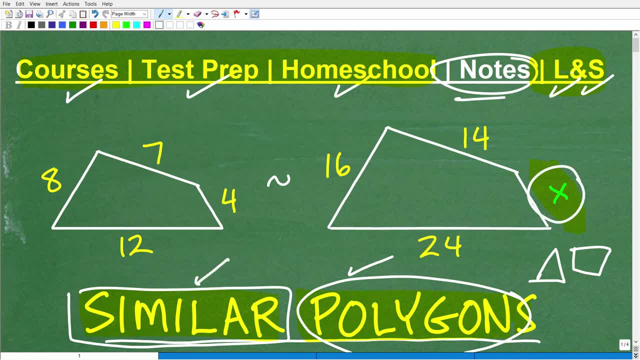 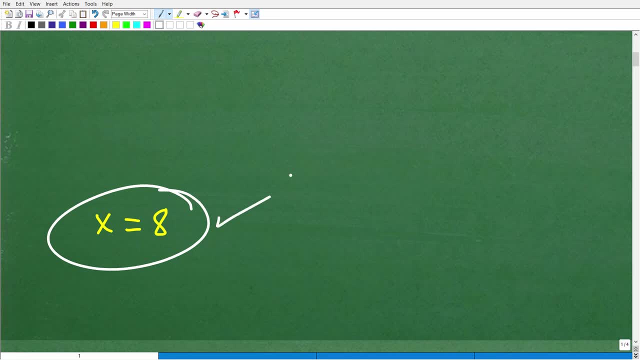 hold off on similarity. but let's show you the answer. We're trying to determine this length of these similar polygons, and the length of that side is eight. So again, you probably you know a lot of you out there- could just use common sense. You're like I don't know what a 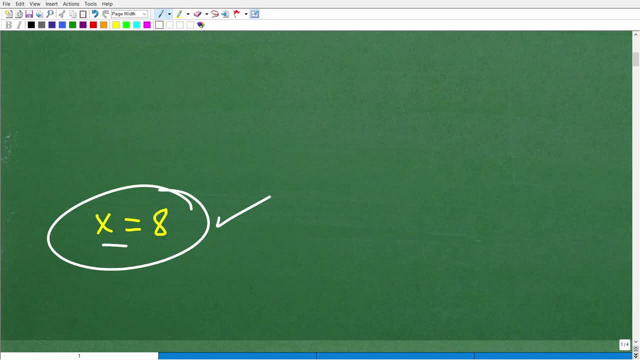 similar polygon is, but just looking at the figure it looks like that side would be eight. If you got that right, let's go ahead and celebrate your success in math by giving you a nice little happy face, an A plus a 100% and multiple stars So you can share with your friends and families that. 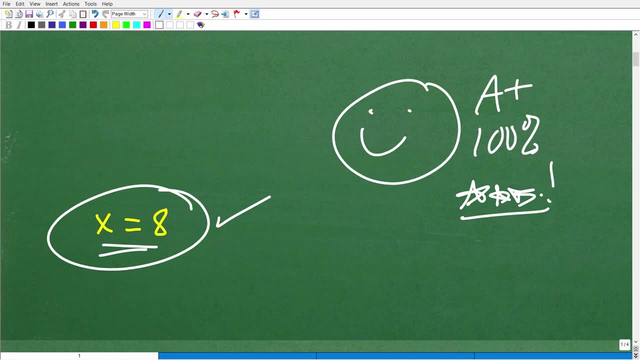 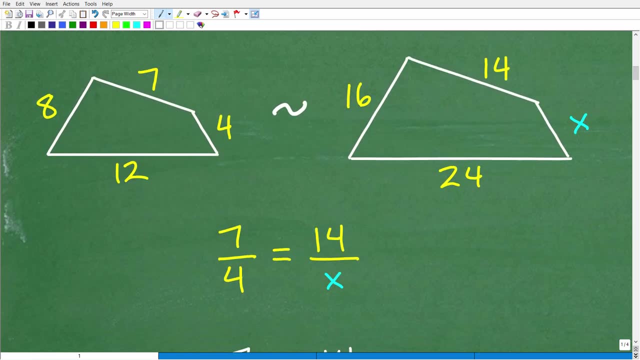 you were able to figure out a similar polygon problem today. All right, so nice job. Let's go and take a look at this figure here and let's just kind of like stop and think about it. So, as I indicated, this is the definition for similar. I already 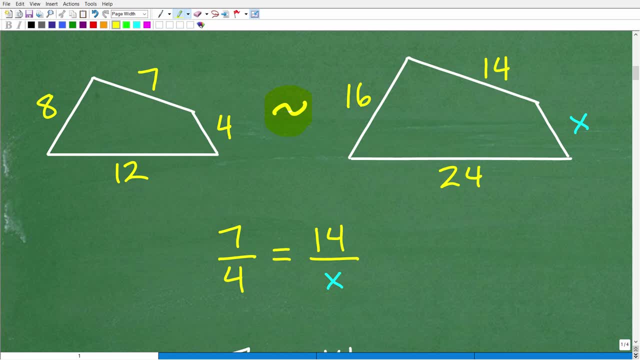 kind of told you roughly what a polygon is. Let me tell you what similarity means. So if you notice, here these basically look like the same shape. This is just a small version of it, This is a bigger version of it, and that's effectively what similarity means in geometry. Okay, it's basically. 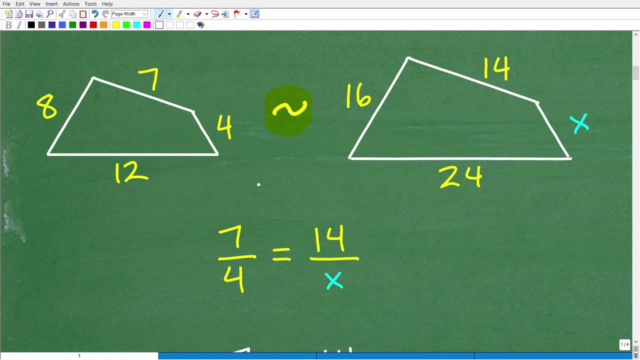 the same shape but different size. I kind of like to think of it as a zoom or out situation, right? So let's suppose you know you were able to kind of grab this, maybe like with your mouse cursor, and then you kind of grabbed this like so, and then you pulled. 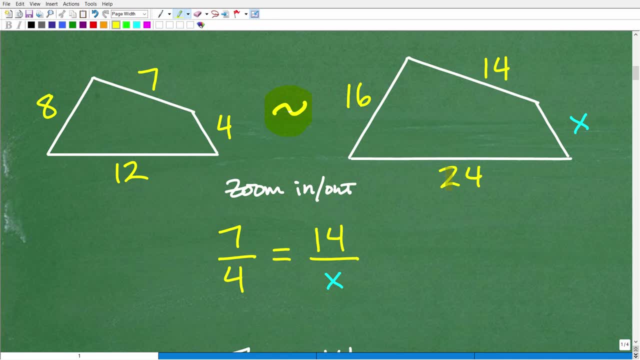 it out and you made it bigger, like this, with your mouse cursor or, you know, maybe with your hands if you're on a tablet PC. That's effectively similarity, Okay, so basically we have the same shape, We just made it larger, or we took the larger shape and made it smaller, Okay that. 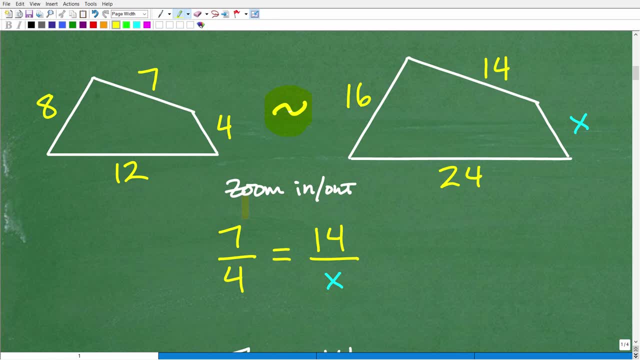 concept in geometry is called similarity. Now, here, this angle would be the same as this angle. Okay, once we kind of change this figure from a smaller to bigger or bigger to smaller, the angles would be the same. Okay, if we kind of notice here, the angles don't change. The only thing that changed here was the 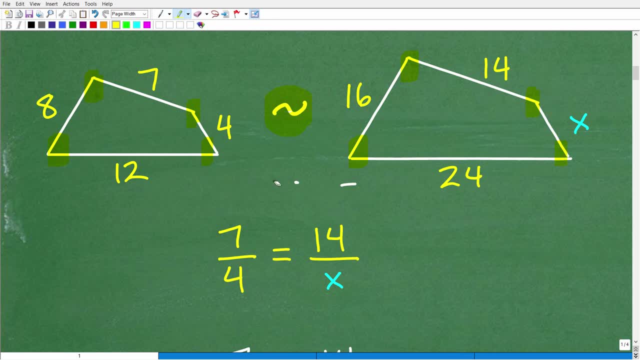 lengths. Okay, but here is the deal right. So when you have two similar figures in geometry, the corresponding size are proportional or corresponding sides are in proportion. So what does that mean? Well, if we take any two sides and we create a ratio, in other words we compare any two sides, let's suppose 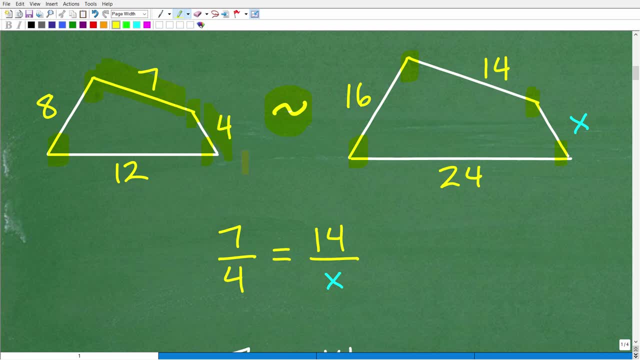 we take this side here, seven, and we compare it to four. In other words, we just create a fraction: seven is to four. Well, that's going to be the same as if we can compare the same corresponding sides. Now, what's the corresponding side? Well, seven corresponds to this. 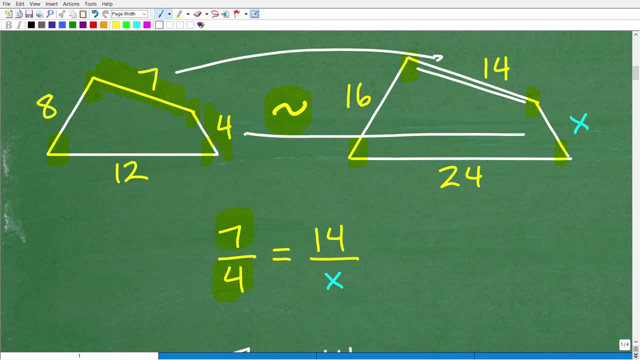 right here with the 14, and the four corresponds to the x. So if I take seven and divide it by four, it's the same as taking 14, or it's going to be equal to 14 to x, right, So effectively. 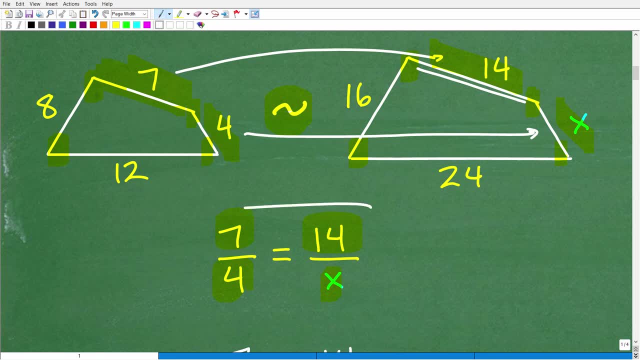 these sides corresponding sides are in proportion. So in other words, we can set up a proportion to solve this problem. Now a lot of you are like saying that is like way too much work. Mr YouTube Math Man, because I just kind of noticed. 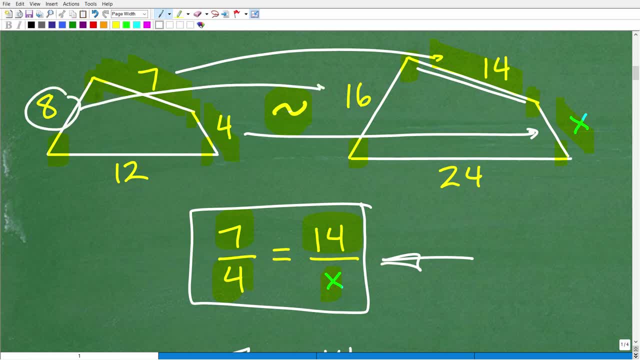 here that eight. when I multiplied it by two, I got 16.. 12,. when I multiplied it by two, I got 24.. And I said: you know what? let me see, seven times two, I got 14.. So probably. 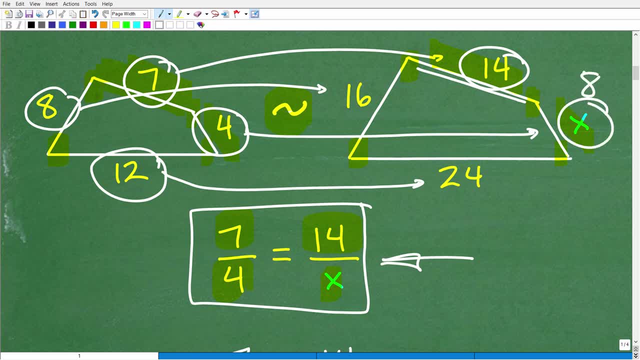 if I took this four, multiplied it by two, I would get eight over here. So again, if you just looked at that and you're like I don't know what similar means, I don't know what polygon means, but I bet you this answer to this is eight, that's good stuff, right? In other words, 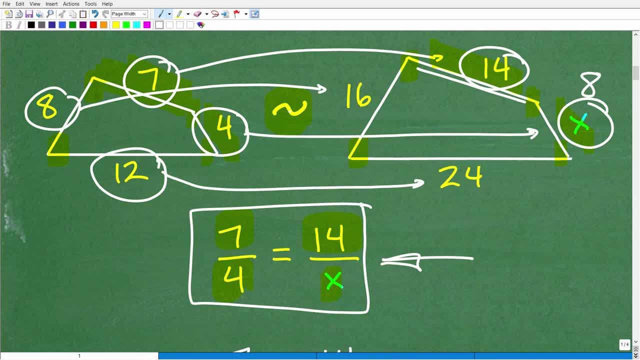 yes, very, very good. It just, you know, is to show that you should never not try to figure out a math problem. Never just look at a math problem and be like, oh, I have no idea. At least attempt it and reason through it with whatever logic you. 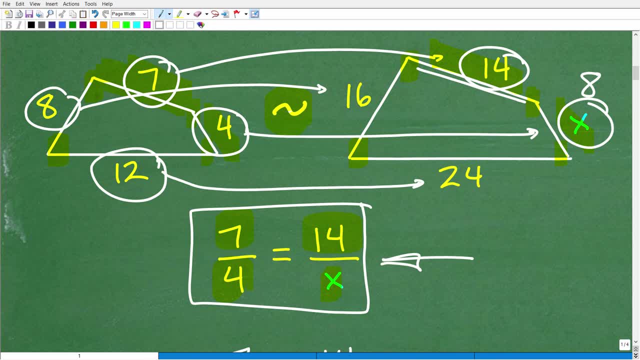 might think is sound, And of course you know we'll have to take a look at your answer. But if you figured that, if you figured out the problem this way, that's perfectly fine. But you need to understand the bigger picture here that we are talking about proportional sides. okay Now 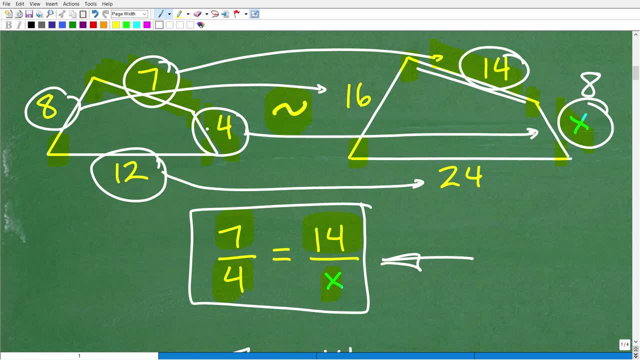 this is an easy problem. I could have made it much more challenging, much more interesting, But anyways, with that being said, all we have to do is figure out this proportion. ie solve for x and we will have gotten our answer. eight, So we have seven over four, is equal to 14 over x, So 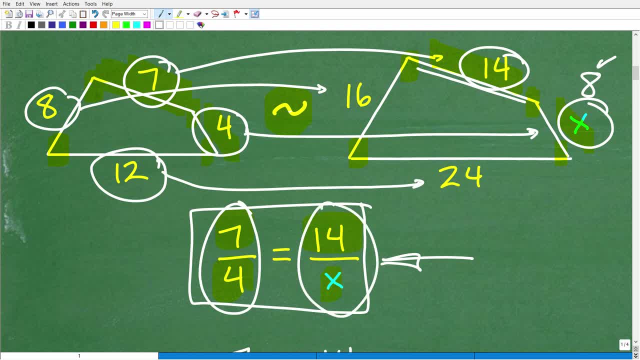 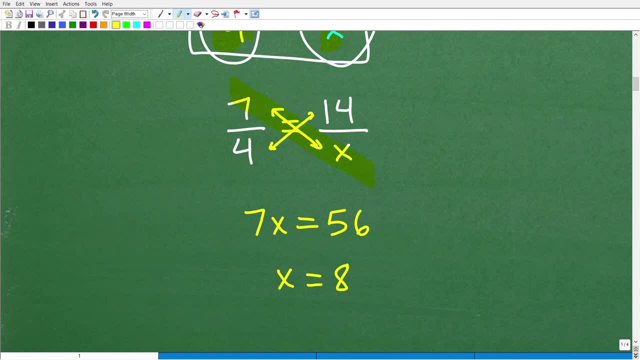 this is a proportion, ie two equal fractions in algebra. So how do you solve proportions? Very easy, All we need to do is use the cross product. In other words, if we multiply across seven times x, that's going to be equal to four times 14.. Four times 14 is: 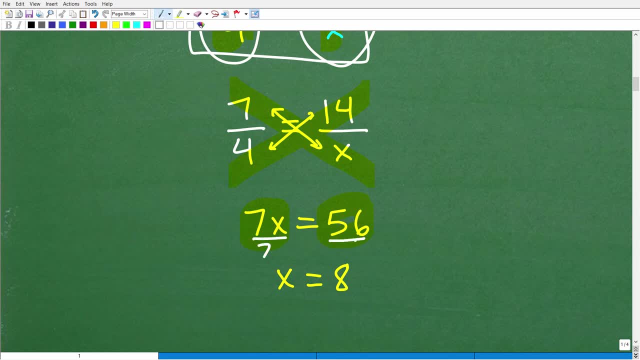 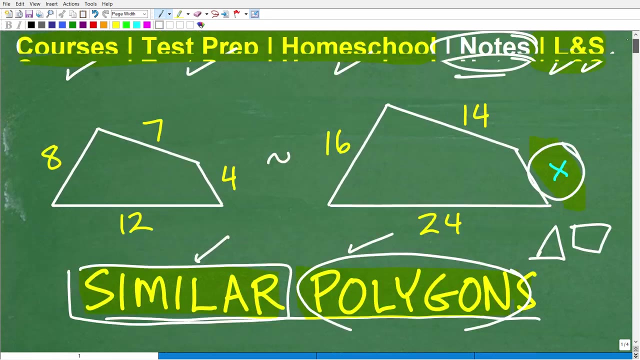 56. And so to solve for x, all I need to do is divide both sides of the equation by seven, and 56 divided by seven is eight. So there is our eight. our missing length: x is equal to eight. Okay, so again, similar polygons. This is not to be confused with a concept of congruency. 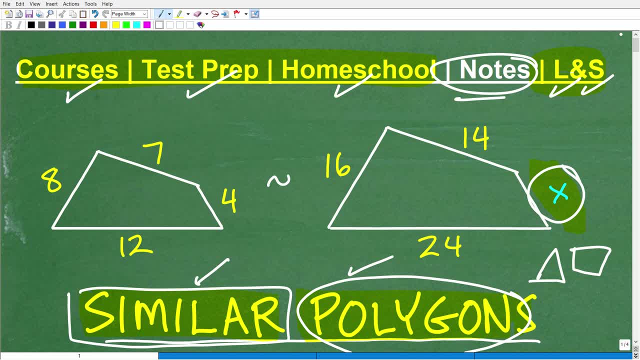 So if you're taking high school level geometry, I have a full, complete high school level geometry course, okay, you might be interested in. And similarity comes up. there's similar right triangles which are, I think, a little bit more challenging than similar polygon problems. So there is, you know. 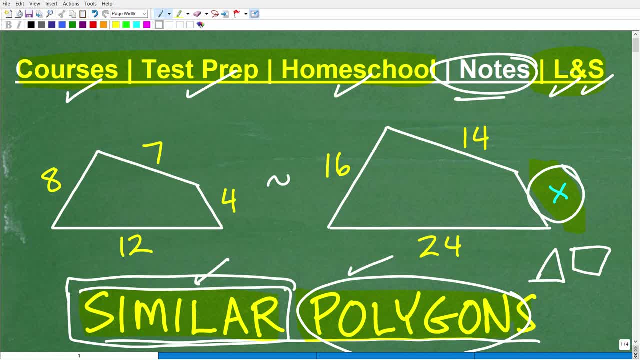 this is a big topic you need to know in geometry. Okay, so don't walk away from me and be like, yeah, I'll never see that again. Well, if you are studying high school level math, you will definitely see similar polygon type of problems. Okay, so hopefully this little video. 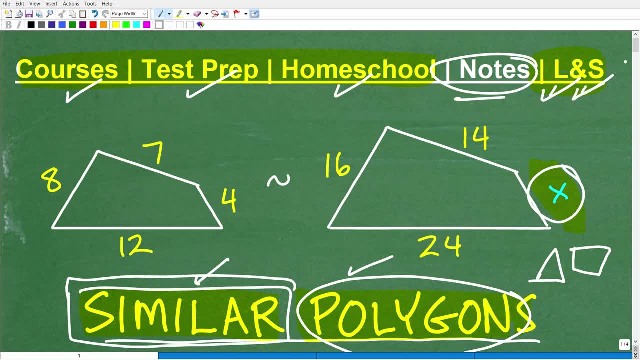 helped you out. If that's the case, don't forget to like and subscribe And, with that being said, wish you all the best in your mathematics adventures. Thank you for your time and have a great day.